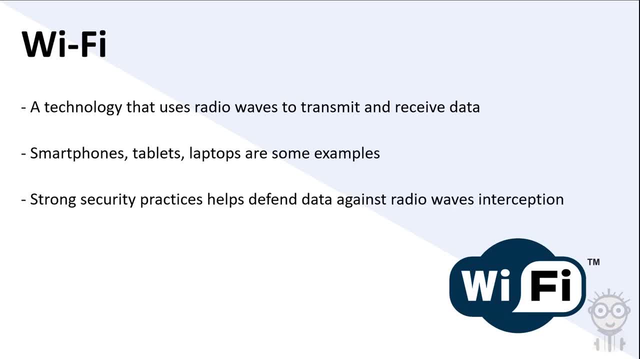 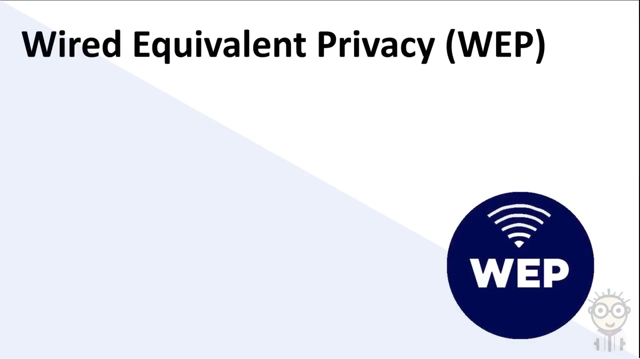 Since Wi-Fi devices use radio waves, these could easily be intercepted by hackers, And so it is important that devices using Wi-Fi are properly configured, using an appropriate set of security standards and protocols. So let's begin talking about the first wireless security protocol, which is Wired Equivalent Privacy, or short for WEP. 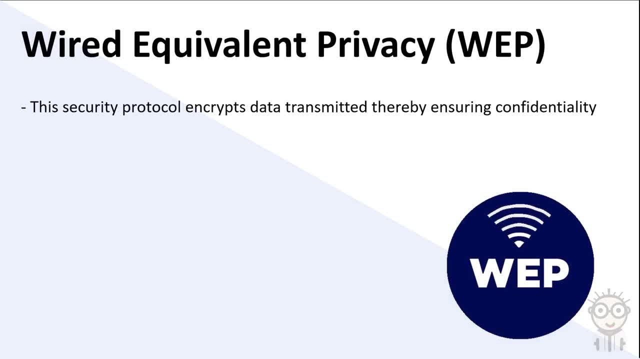 This security protocol encrypts the data transmitted by wireless systems and ensures that confidentiality is maintained. However, it does have security flaws, One such being its short key strength of 64 bits, Or sometimes 128 bits, makes you vulnerable to hackers, who, in fact, have exploited this protocol. 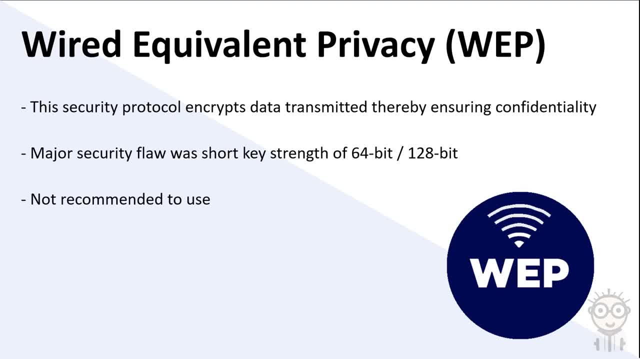 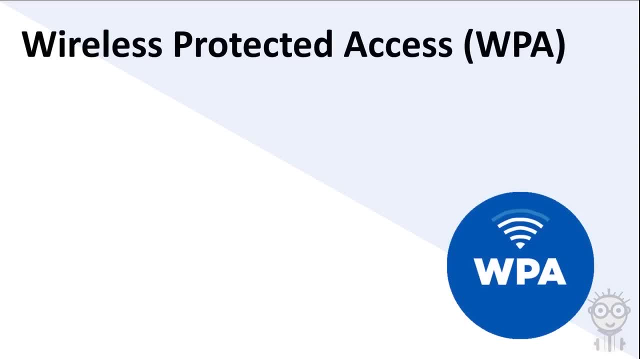 So this standard is not recommended anymore and must be replaced. Luckily, one that did cover many of the WEP vulnerabilities was developed, and this was the Wireless Protected Access, or WPA. This security type did offer some improvements, such as its handling of security keys. 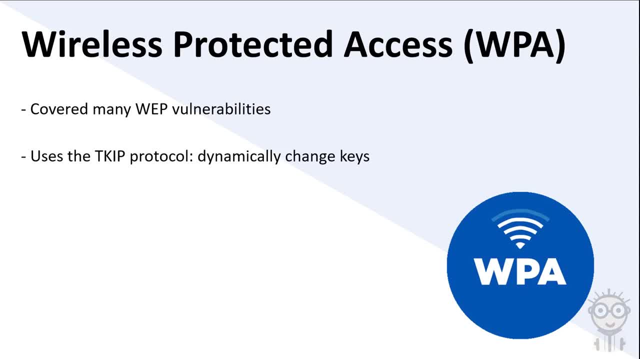 For instance, it used the Temporal Key Integrity protocol to dynamically change the keys the systems use. This feature was not present in the Wired Equivalent Privacy. Another improvement was its key size, this time using 256 bits. One commonality, however, between both of these protocols was the use of RC4 screen cipher. 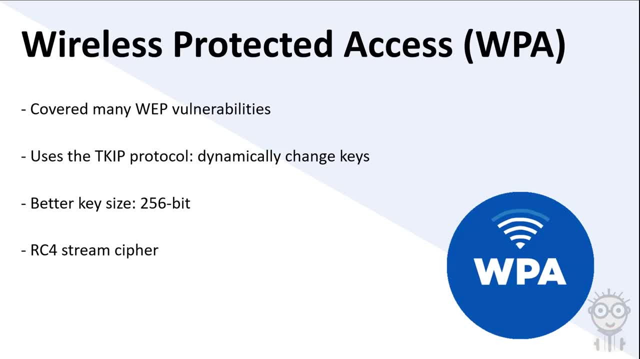 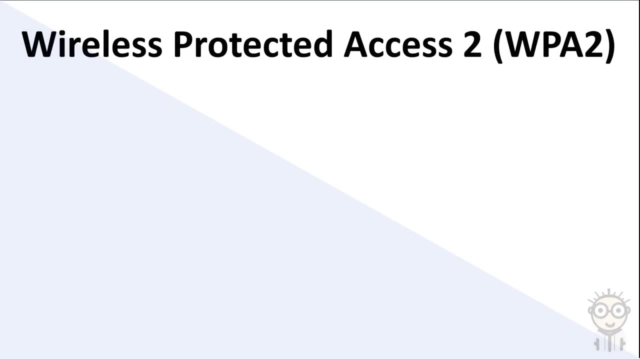 Despite these improvements, the WPA was still exploited and hence was no longer recommended and needed to be replaced by stronger protocols, So the next upgraded version of WPA was developed and adapted. This was known as the Wi-Fi Protected Access 2.. 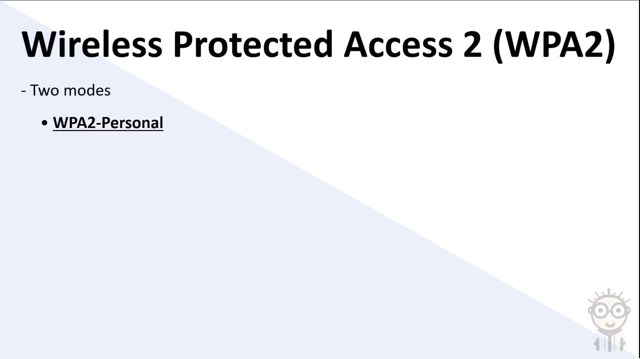 This standard comes in two modes: the WPA2 Personal and its Enterprise. WPA2 Personal is known as the WPA2 PSK. PSK is standing for Pre-Shared Key, meaning its authentication is based on the pre-shared key, allowing home users to manage the keys. 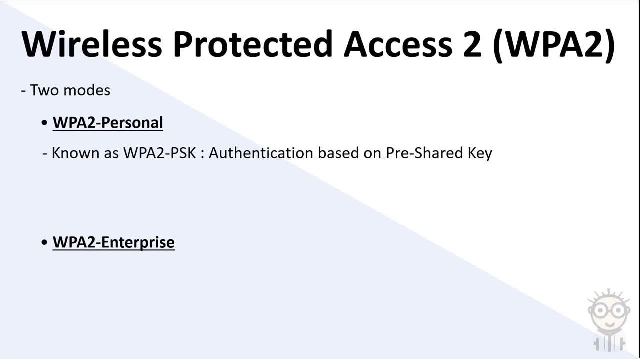 Here the router is given the pre-shared key, which is basically the passwords. It then uses the Temporal Key, Integrity protocol or Advanced Encryption Standard, depending on the encryption selected, to combine the password with the service set identifier to generate unique encryption keys for each wireless client. 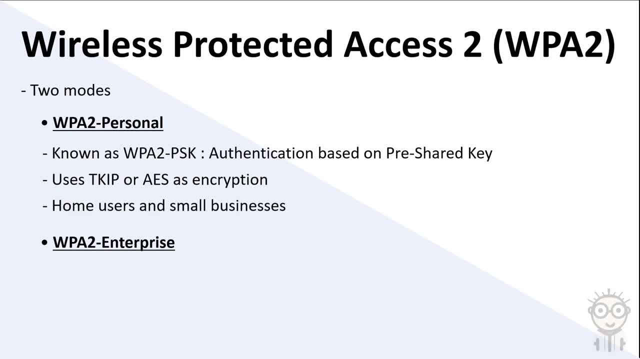 Most users and small businesses even deploy WPA2 Personal as a standard Wi-Fi security type. Another of its modes is the WPA2 Enterprise. Here, each user of the wireless network has either their own unique username and password or a certificate installed on the device. 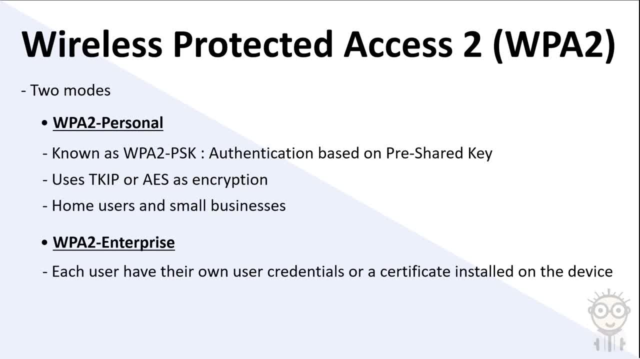 Since each user has a unique logon, it is easier to revoke the permission of individual users without having to change the common pre-shared key, like the one in Personal mode. WPA2 Enterprise uses the 802.1X protocol to authenticate connections. 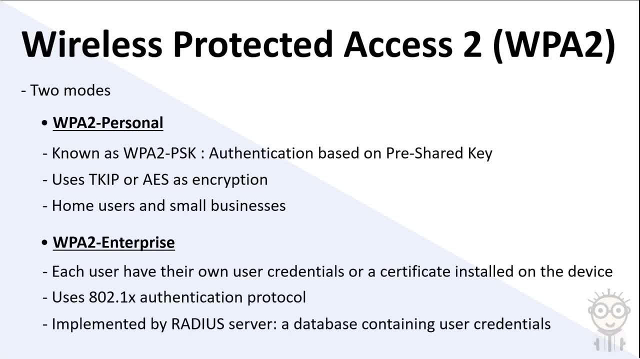 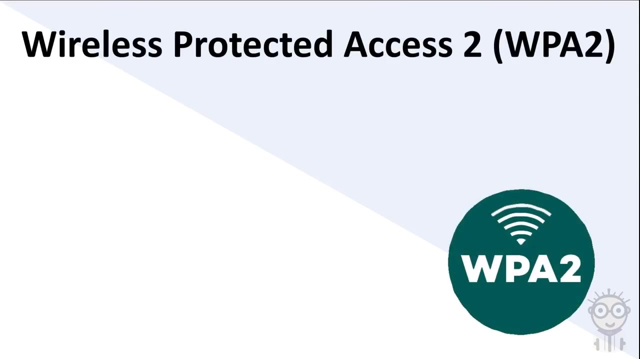 and a remote authentication dialing user service server is required for implementing WPA2. Enterprise RADIUS is basically a database which stores each user's credentials. This functionality is quite complex to use in, hence more smaller networks with WPA2 Personal. It is, however, important to note that both of these modes use the Counter Mode: Cipher Block Chaining Message Authentication Code protocol. 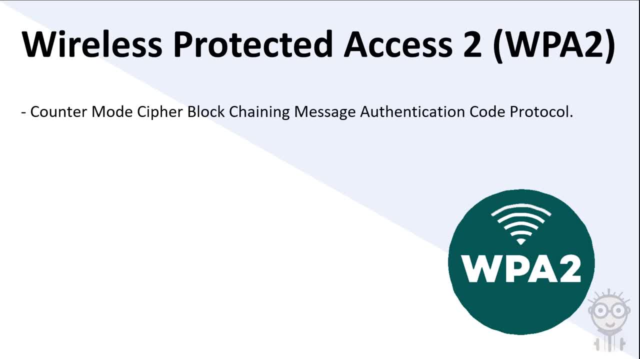 also known as CCMP protocol, and is based on the Advanced Encryption Standard algorithm, which provides message authenticity and integrity verification and is much more reliable than TK IP. WPA2 was able to fix many of the vulnerabilities in WPA and continues to remain a standard for many years. 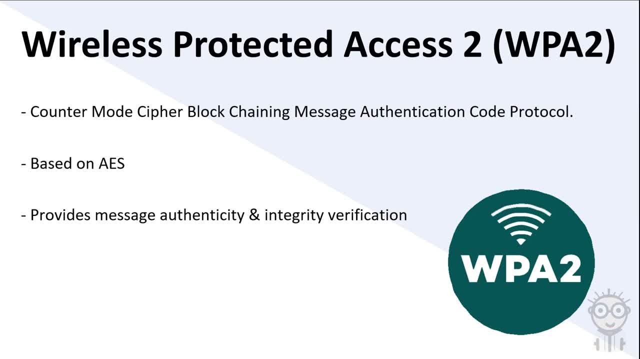 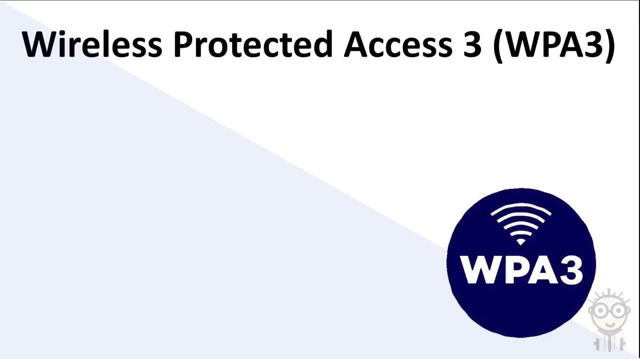 but it too, however, fell short of vulnerabilities, resulting in the development of even upgraded version, known as WPA3.. This successor, developed in 2018, improves security of encryption by using simultaneous authentication of equals in place of the PHP authentication mode. 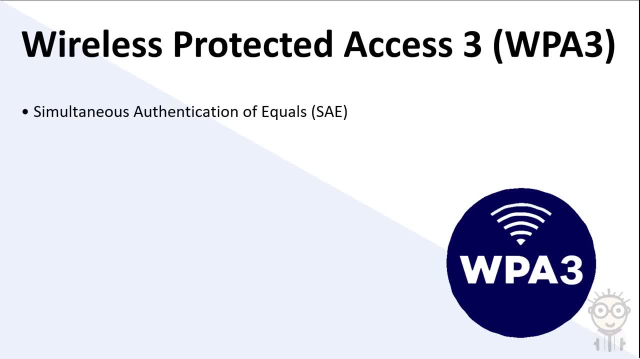 Simultaneous authentication of equals is basically a password based key exchange method that uses a Dragonfly protocol to perform the key exchange. It helps create a strong shared secret for securing data and is extremely resistant to offline dictionary attacks. WPA3 also comes in two modes: Personal and Enterprise.